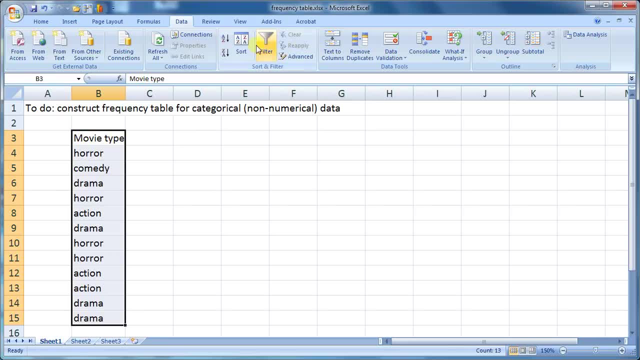 need to include the column header, not just the data itself, and then you say filter. okay. after that you say advance because you're gonna. you want to build a list, so you click on advance. you already filter the list, but this time we are going to copy to another location. the list range is already there, including the column. 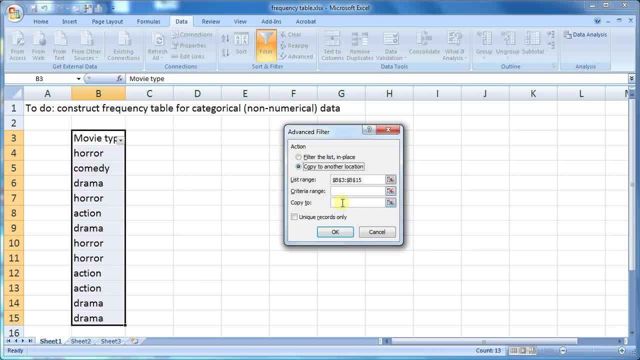 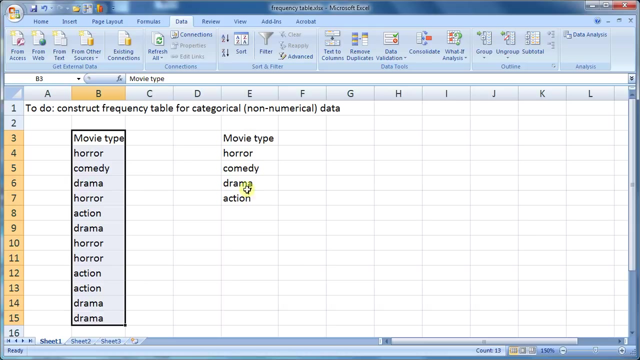 label. and then you want to tell Excel to copy, to like this location, this new location where you have a unique record of each data. so you would have only one horror, one camera comedy here. and then you say, okay, see how we will have another list with the all the classes list. 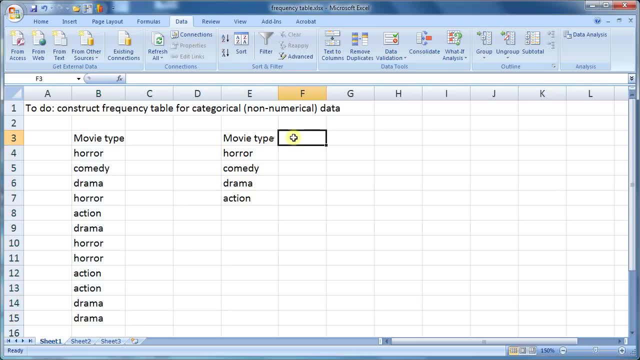 only once. then we will try to build a frequency. now, instead of using equal frequency here, we'll use equal count. if to do that we again, we select all the frequency entries or the cell in the frequency column that you want it to count, and then you move your cursor back. 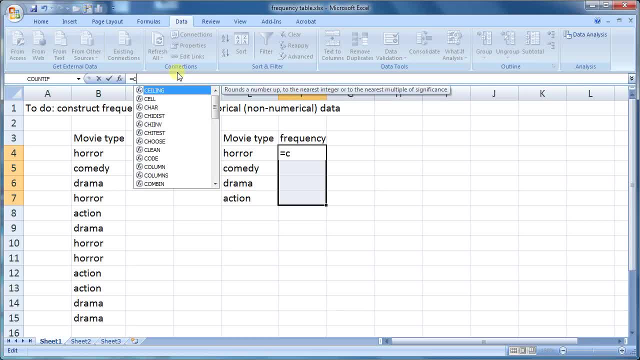 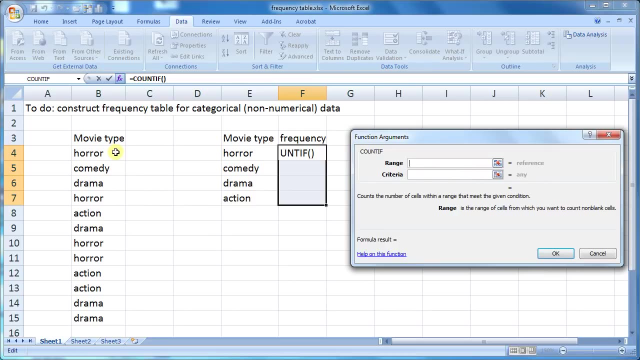 back to the formula bar and you type equal count. if I do ctrl a to get the input prompt, then for the range of data, this would be the range of data value now in this time. this time we do not use the movie type, we do not include the 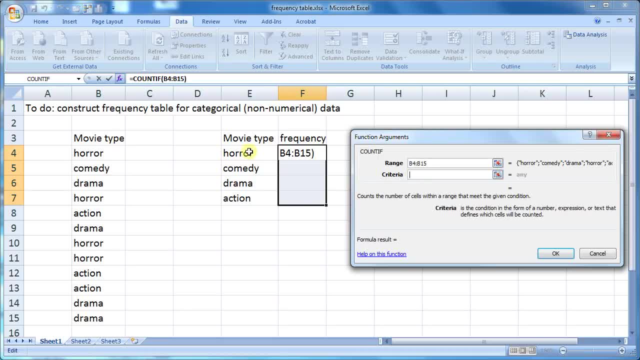 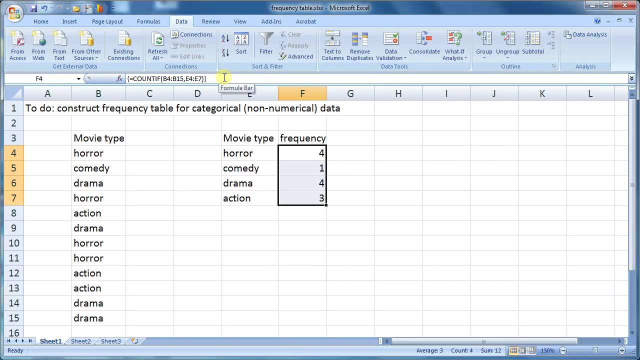 column header. the criteria would be the classes. again I we do not include the movie, the column header also. and after that we move our cursor back to the formula bar, press shift, control down, shift and control down at the same time and then press ENTER. and that's how we build the frequency table. 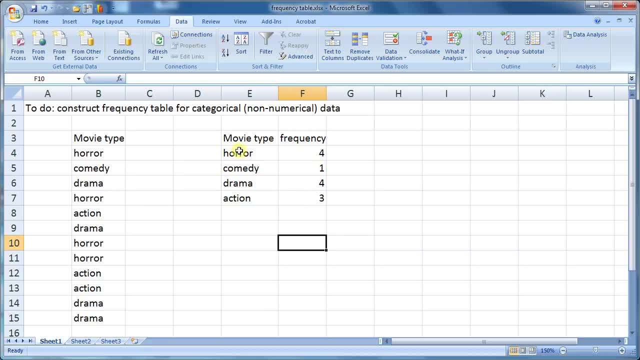 so. so this list that tells us that there are four occurrence of horror, one occurrence of comedy in the original data, etc. etc.